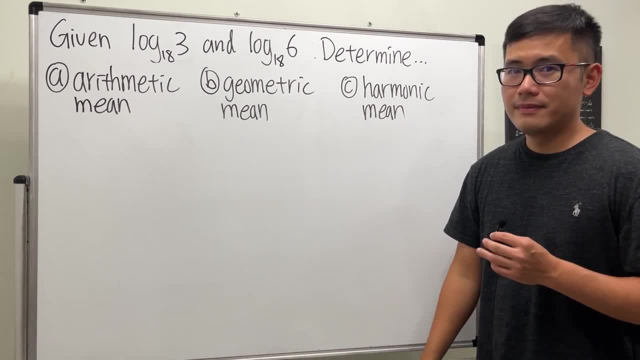 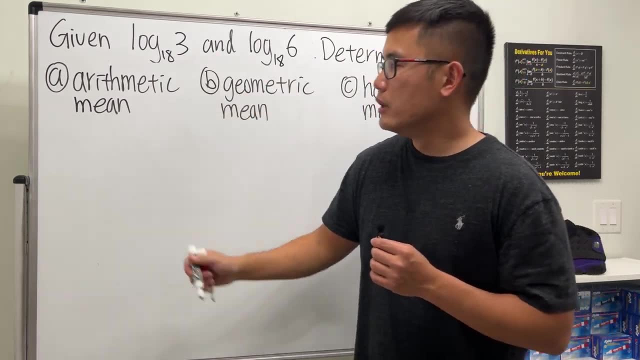 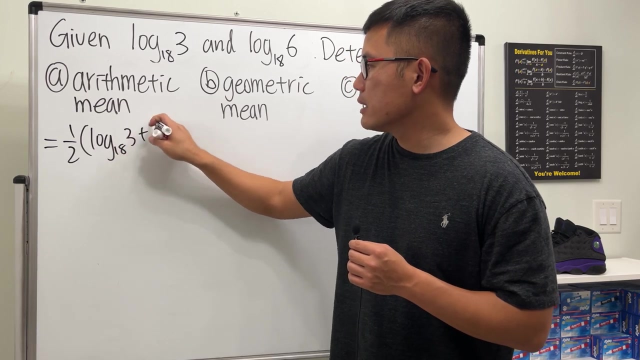 please pause the video and try this first. Done. Okay, here we go, For the arithmetic mean for two numbers. we just have to add them up and then divide it by two. So we can also say that one half times this plus that, namely log base 18 of 3 plus log base 18 of 6.. And when we add these two? 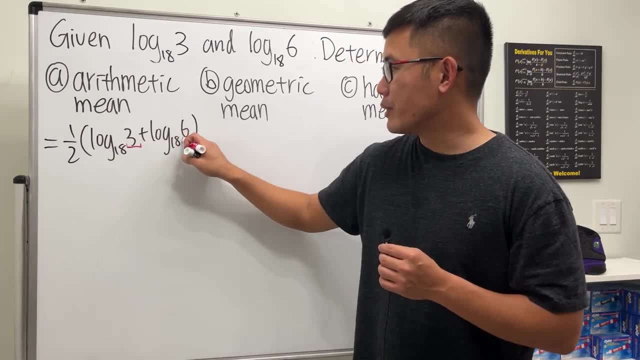 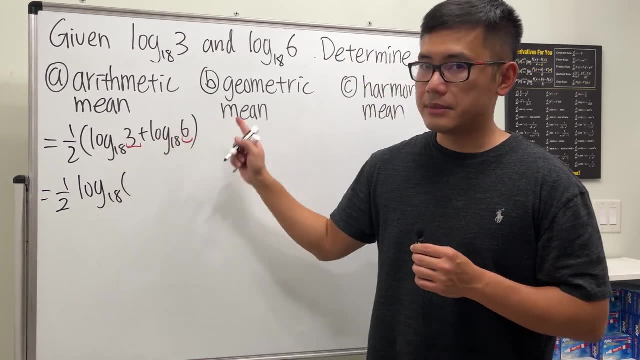 logarithms. when they have the same base, we can just multiply the numbers inside. So this is the same as one half times log base 18, and that's 3 times 6, which is 18.. And log base 18 of 18 is. 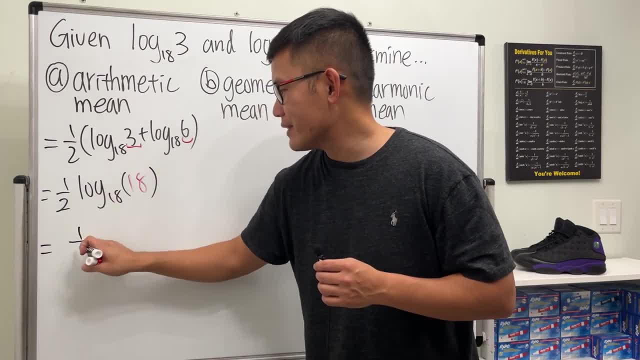 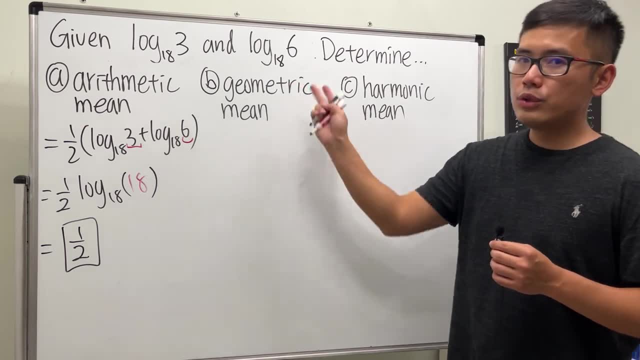 just equal to 1.. 1 times one half. yes, it's just one half. That's pretty cool. Now let's look at the geometric mean. This right here: when we have only two numbers, what we have to do is multiply them and then take the square root. If we have, 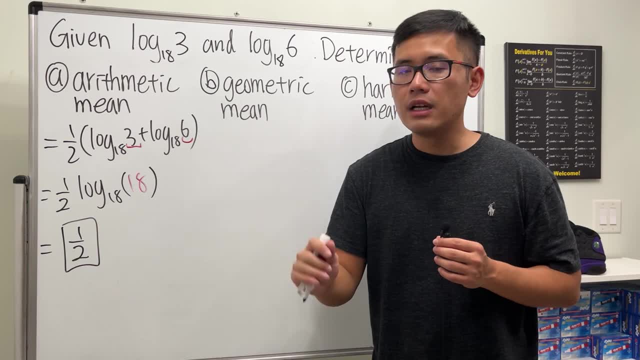 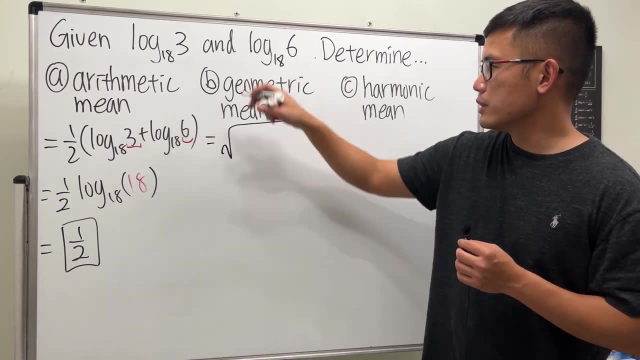 five numbers, then we will multiply all those five numbers together and then take the fifth root, et cetera, et cetera. So for this right here we will get the square root and then we just multiply log base 18 of 3 with log base 18 of 6.. 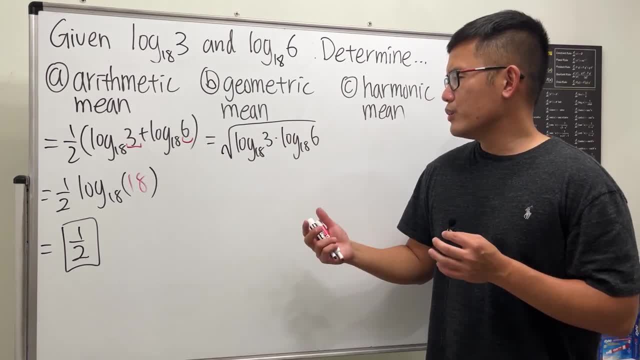 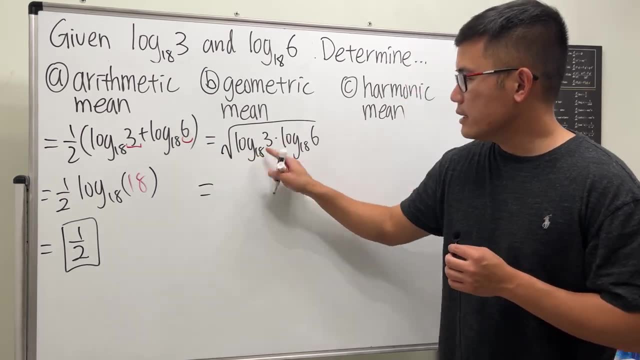 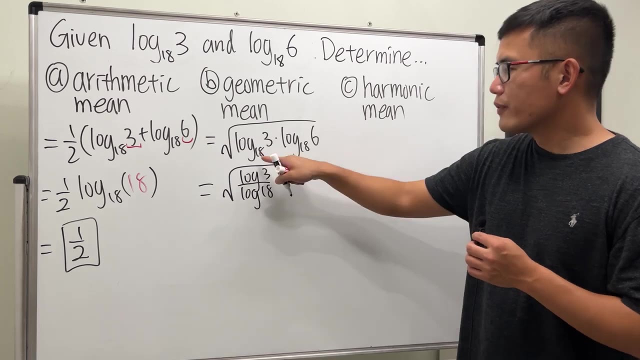 Unfortunately for this right here we can't really do anything nicely. We can use the change of base formula. that's about, so let's go ahead and do that- And that is to write this as log of 3 over log of 18.. And of course, you can also use natural log or log base of 7, as long as this and 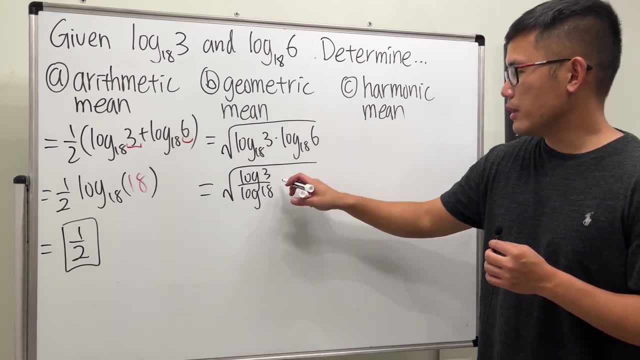 that are the same. that would be okay. And let's also go ahead and do the same thing right here, which is just log of 6 over log base 18 of 6. And that's it, And that's it, And that's it, And that's. 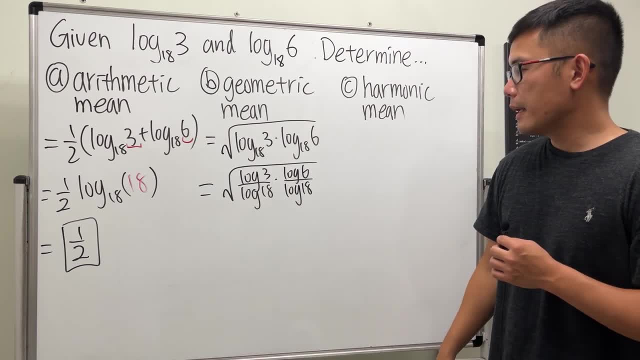 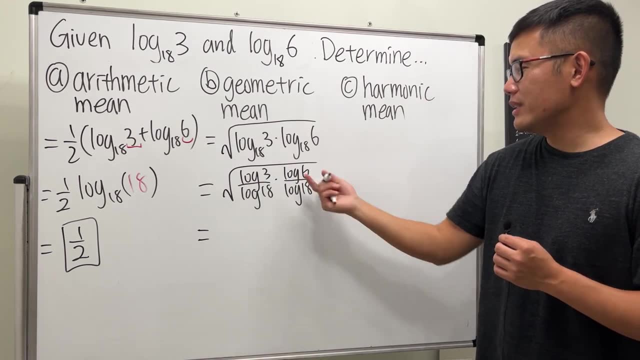 log of 18.. Okay, And then what do we do next, though? Well, unfortunately, log of 3 and log of 6,, when they are multiplying, we can't really do anything, So we'll just leave them in the square. 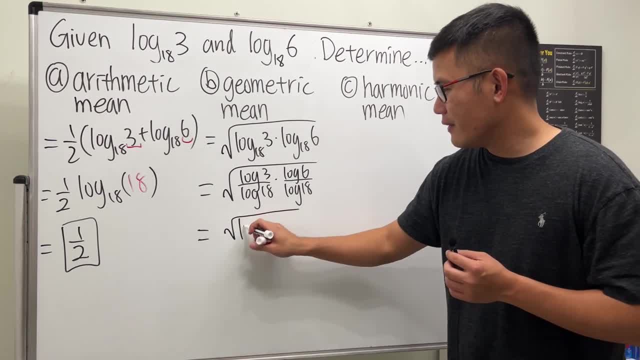 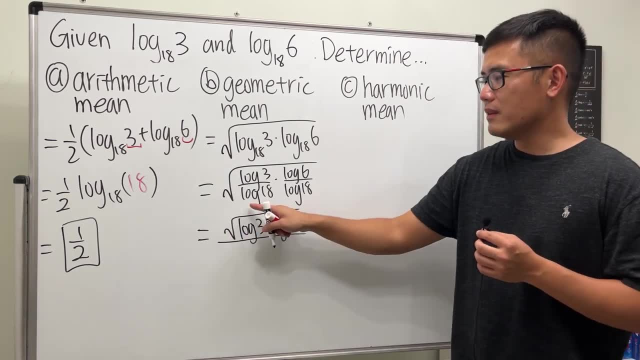 root. I will just write it as square root of log of 3 times log of 6.. But at the bottom, here you see, we have log of 18 times log of 18, which is log of 18 squared right, Quantity squared. 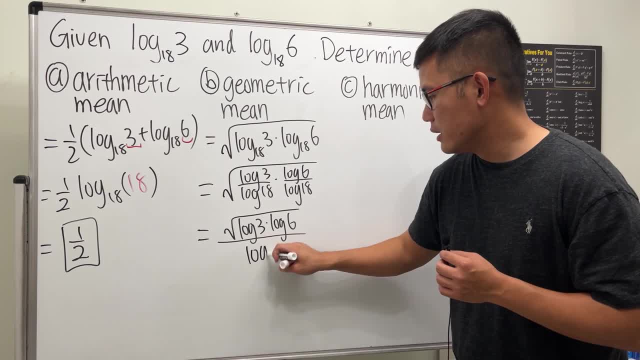 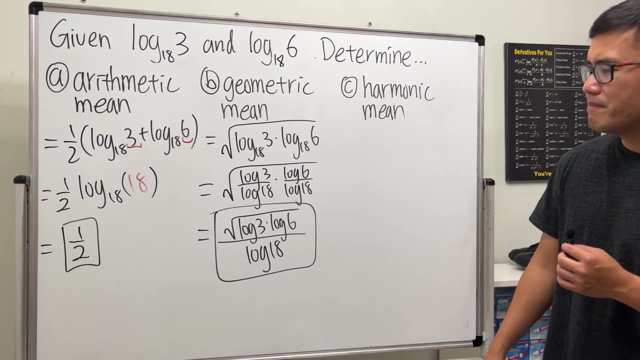 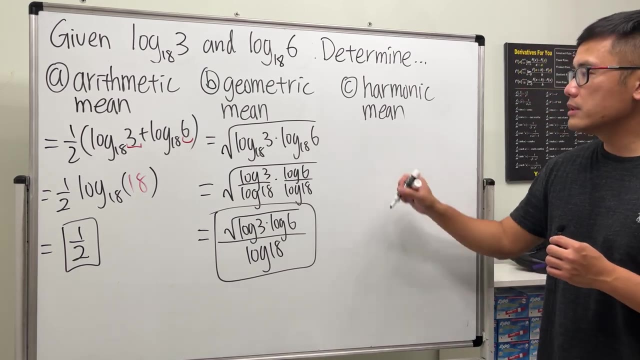 In the square root. so no more square root. So just say this and then log of 18 on the bottom: Yeah, So that will be it for that. And of course, yeah, just leave it like that, Much better. Lastly, the harmonic mean When we have two numbers. then we do the following: 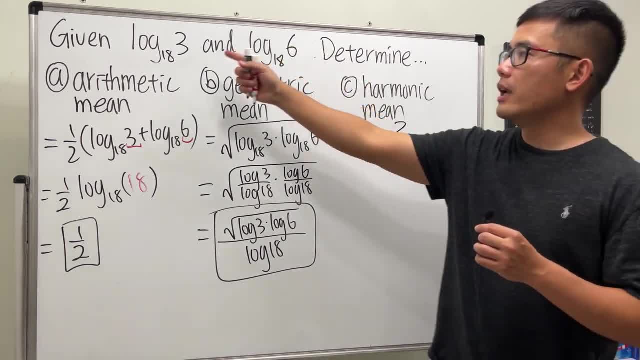 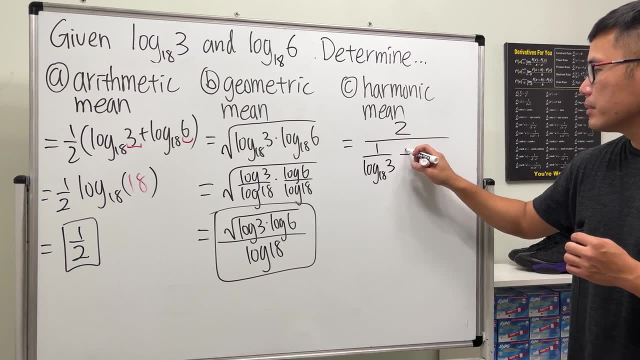 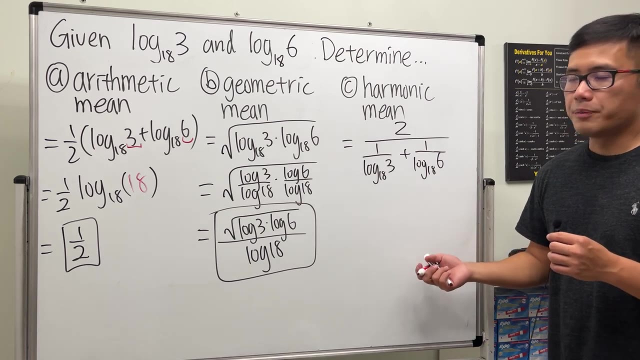 We do 2 over the sum of their reciprocals, And that will be 1 over log of 18 of 3, and then plus Log of base of 18 of 6.. And then let's just go ahead and do a change of base formula. 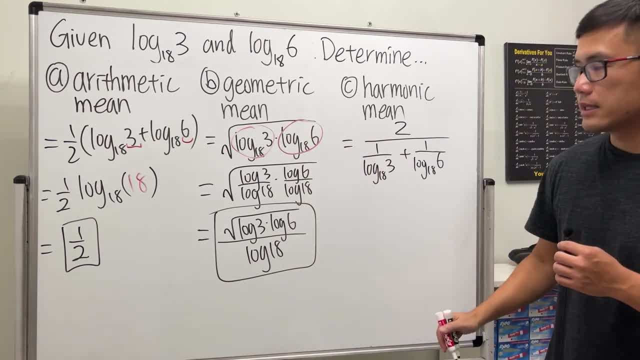 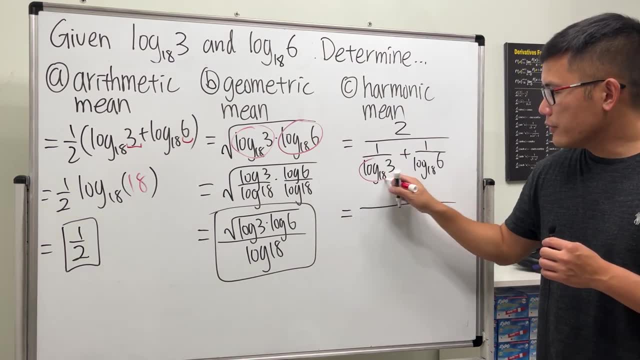 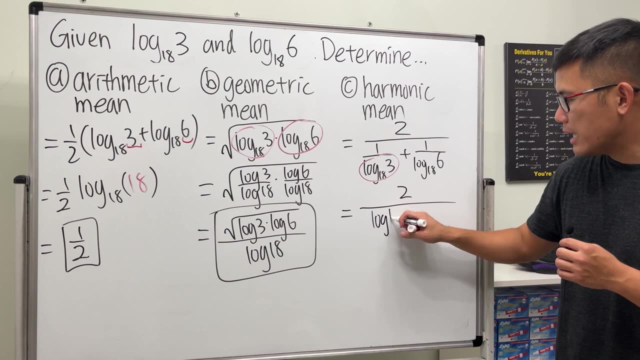 Like I called it earlier, like this is equal to that and this is equal to that. So this right here we will have 2 over well, log base of 18 of 3 is supposed to be that, but it's the reciprocal, So I'm going to write it as log of 18 on the top and then over log of 3.. 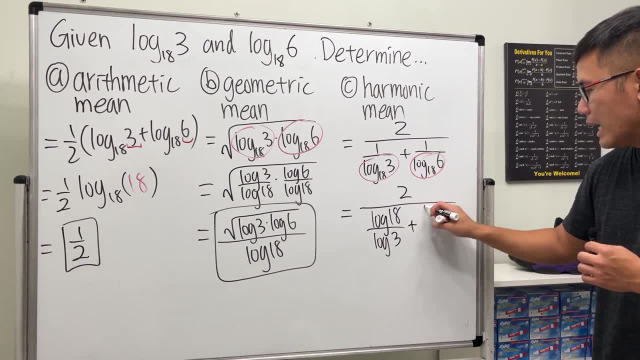 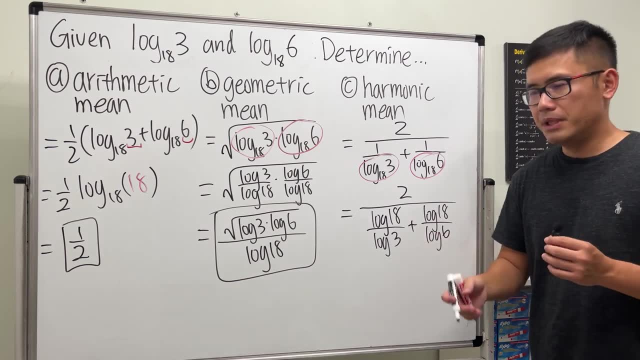 And then for this right here same thing, it's the reciprocal. So we have log of 18, and then over log of 6.. And if you want to use ln, be my guest, right, We will have the same answer at the end, The following: wise, not the expression wise. 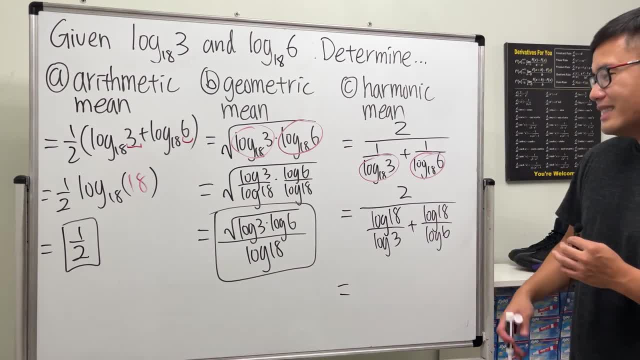 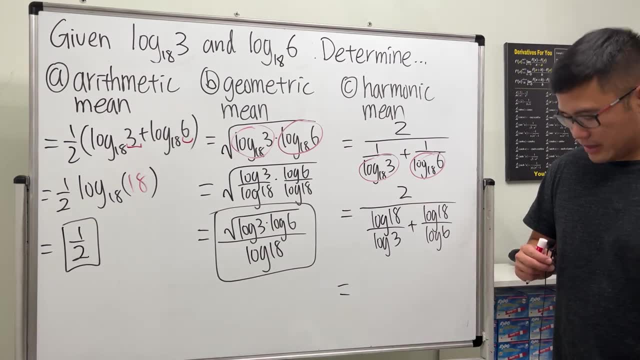 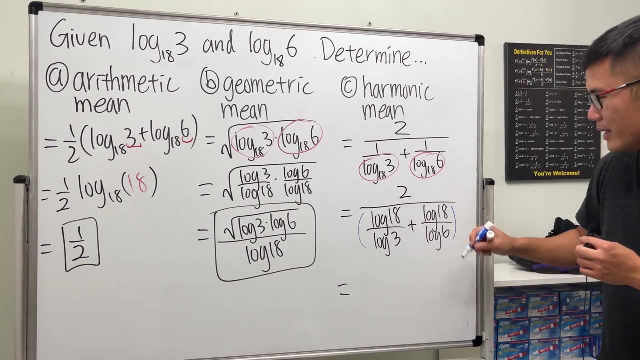 But anyway. so how do we really simplify this? I don't really know. I think I'm just going to take out my blue marker now and then I'm just going to multiply the top and bottom by the denominator. I think that's what I can do. 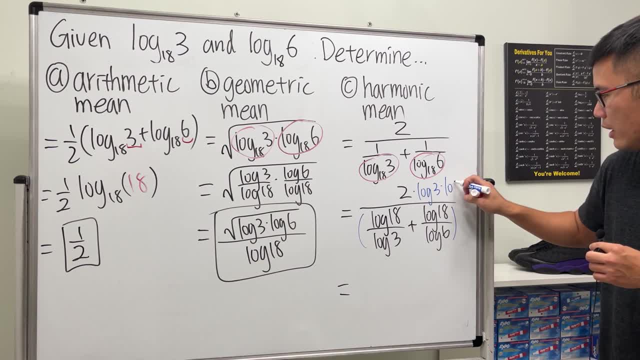 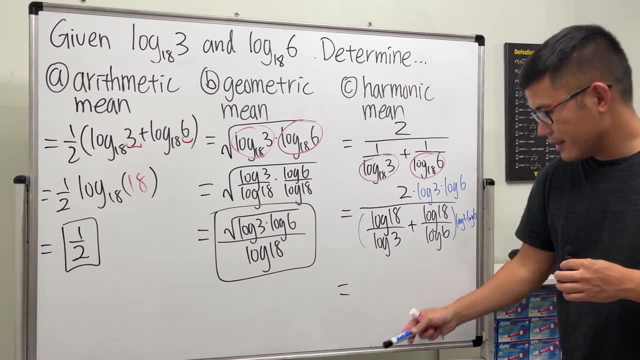 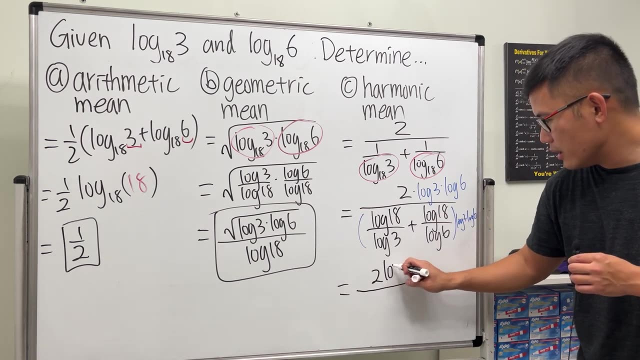 So let's multiply this by log of 3, and then also log of 6, and then let's also do the same here: log of 3 times log of 6.. Okay, and that's about all Okay. so on the top we have 2 log of 3 times log of 6..